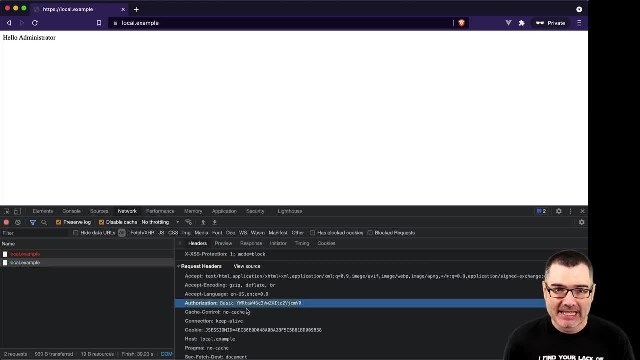 But the value doesn't look like my username and password. It is, but it's just encoded, It's not encrypted. I'll come back to this in a minute, But first let's look at the example, again from the command line. My favorite client is http, but something like curl would work here too. 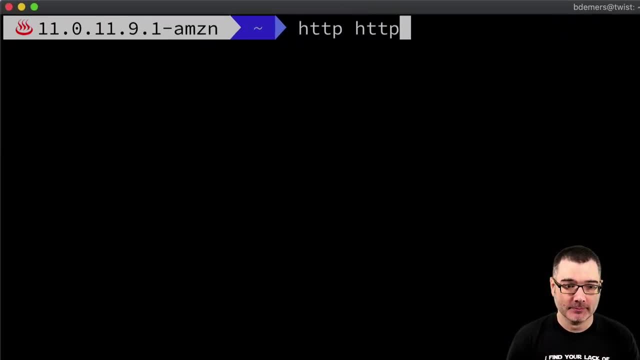 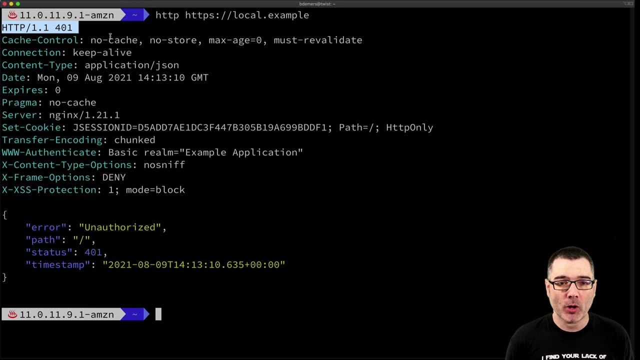 Alright. so, just like before, I'm going to make the same request to my local example, And you can see again that the server responded with a 401.. The important thing to note here is that the server also set a response header. this: 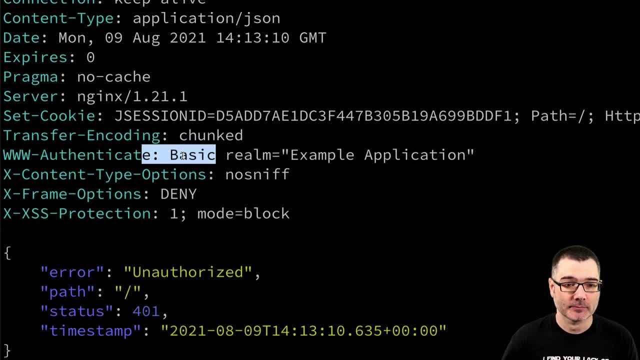 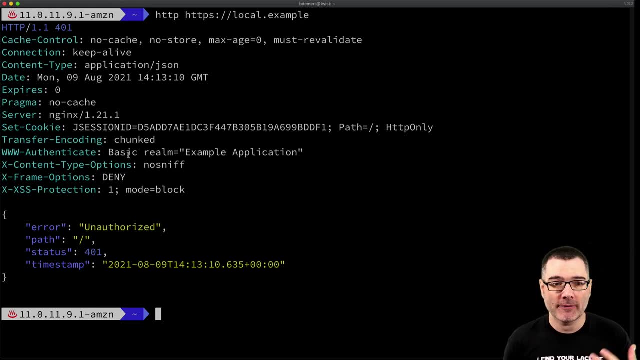 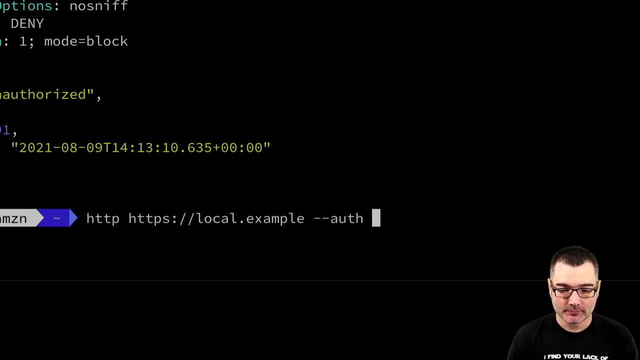 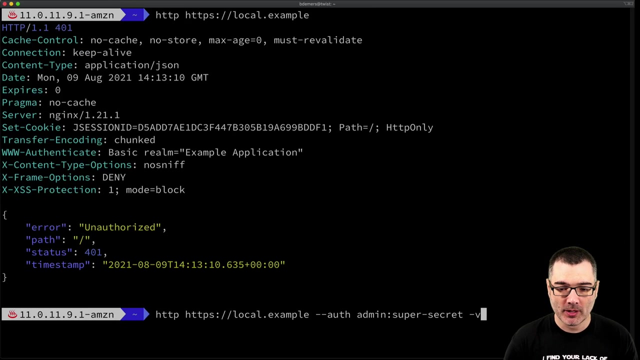 www authenticate basic. This is how the browser knew to prompt me before It sees this value, and it knows to prompt me for username and password. So if I make the same request again, this time with a username and password, I'm going to add the verbose flag so you can see both the request and the response. 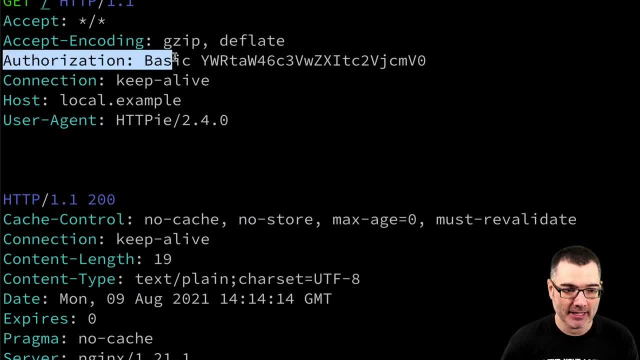 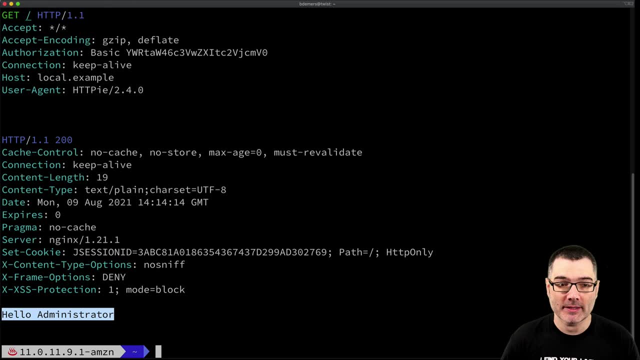 You'll see that same authorization basic header set again with that same value, And this time the server responded with a 200 and a simple hello message. Let's get back to how the username and password were actually sent over the wire. This value in the authorization header is a base64 encoded version of my username. 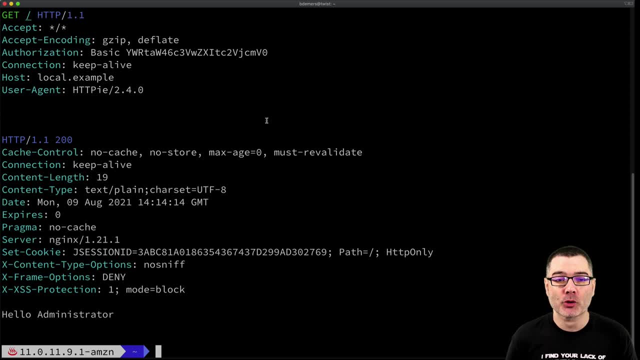 colon password. This value needs to be treated as plain text, as anyone with this value can decode it. I'll recreate this value on the command line, but you can use any base64 tool you want, such as base64 and codeorg. 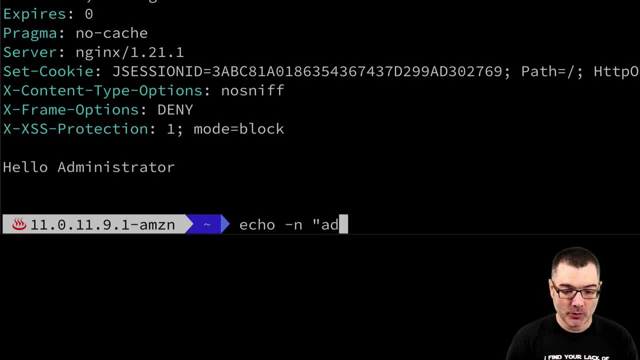 So for this I'm going to use echo and I'm going to use my username, colon password, just super secret, which is still a terrible password. I'm going to pipe that to base64. And I'm going to get back the same value as up here. 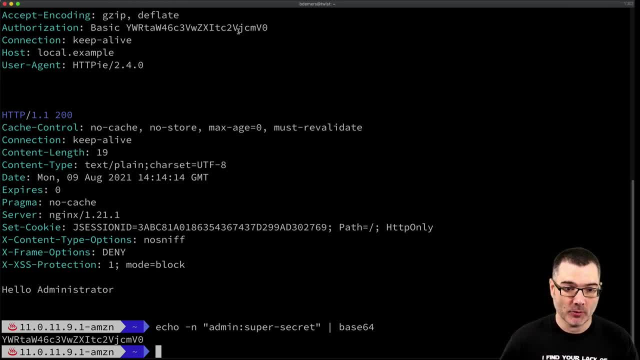 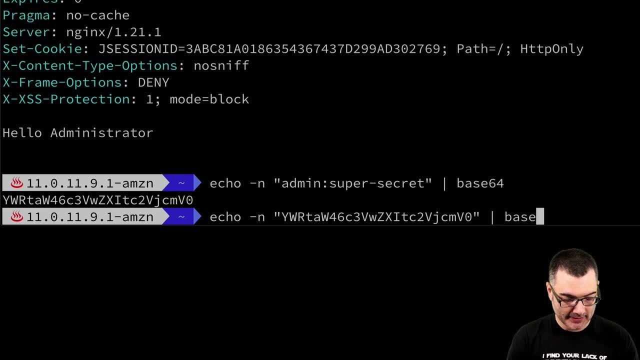 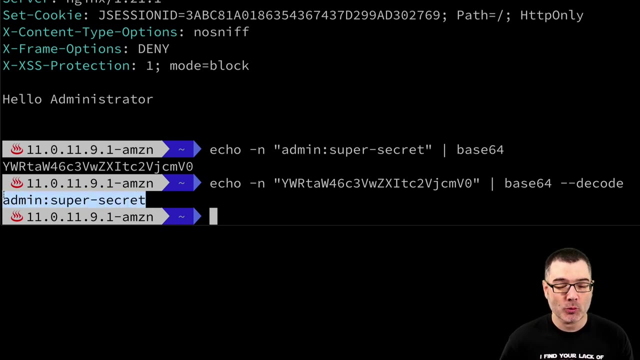 So on the server, the server would decode this base64 encoding value So in echo and we'll send this value to base64. This time we use decode And again we'll get the value out. On the server side, the server would just.